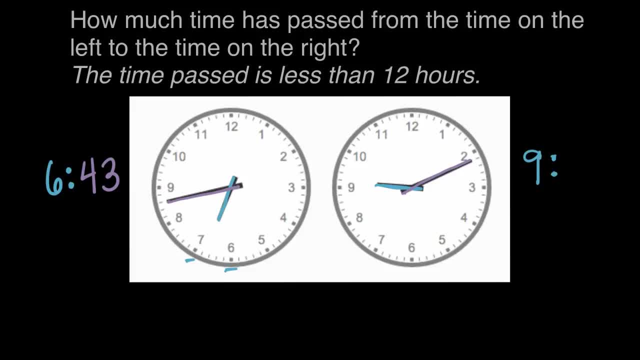 start at the top and it's five, 10,, 11 minutes after the hour on the right. So the clock on the right is 9-11.. And now what we wanna know is: how long does it take to get from this first time? 643,. 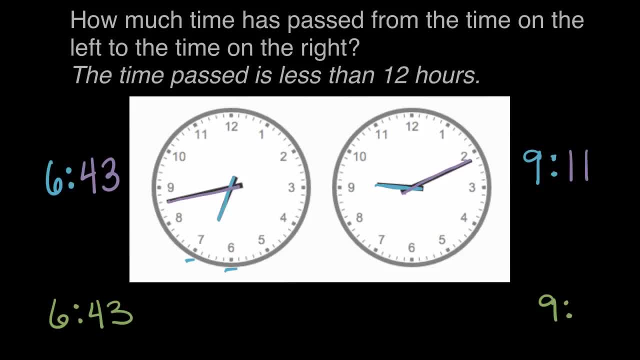 all the way to nine o'clock, And then our minute hand right here all the way to the second time, which is 9-11.. One way we could figure this out is to break it into little parts. Let's first. let's first just see. 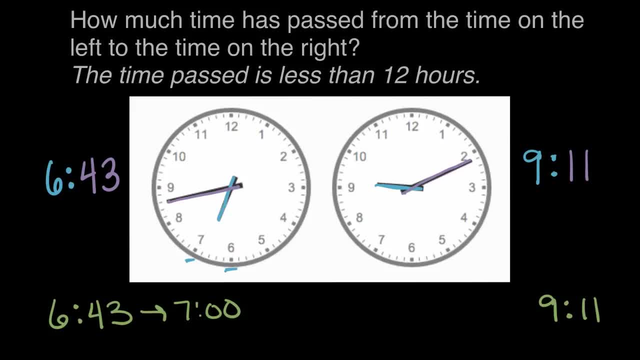 how long does it take to get to seven o'clock? So, on this first clock, as soon as the minute hand gets up to the top, it'll be seven o'clock. Let's see how long is that From here where it is. it has two more minutes. 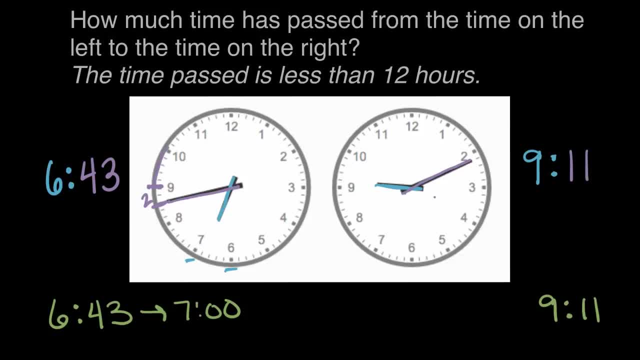 to get to the nine And then from there it has five, 10,, 15 more minutes to get all the way to the top of the clock. So until seven o'clock will be two minutes plus 15 more minutes, or we can write that as 17 minutes. 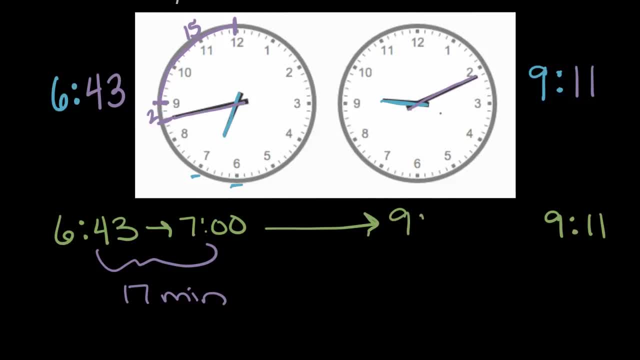 Then from seven, let's stick with the hours for a second. let's just get from seven to nine o'clock. So from seven to nine- at seven o'clock the hand is at the top. it'll go all the way around one hour to be eight o'clock, all the way around. 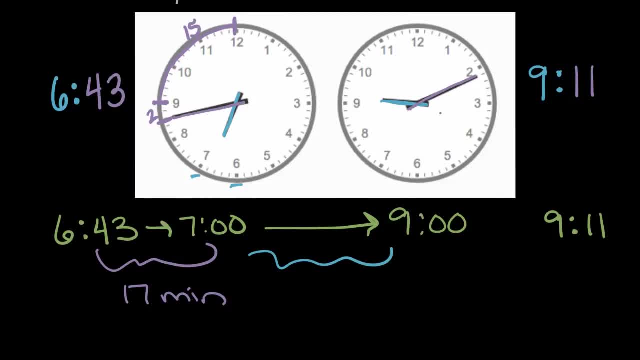 another hour to be nine o'clock. So that's a total from seven to nine of two hours, And then finally from nine until 11 minutes. after nine the minute hand will be at the top and it'll go five, 10,, 11 minutes. 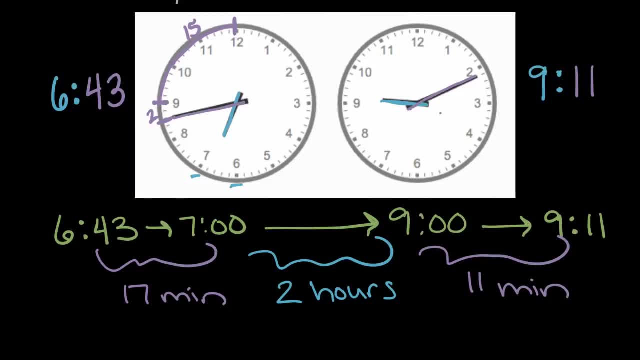 So this will be 11 more minutes. So in total, from 6.43 all the way to 9.11, is 17 minutes plus two more hours plus 11 minutes, So we can write that that's gonna be two hours. 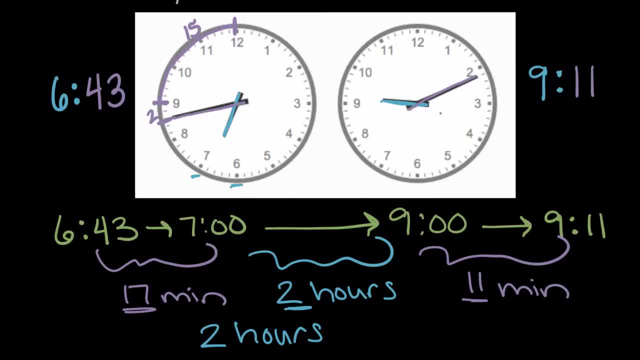 And then we can combine our minutes 17 and 11,, 17 and 11, that will be eight ones, a 10 and a 10 is 20,, so 28 minutes. It takes two hours and 28 minutes for the clock to go from 6.43. 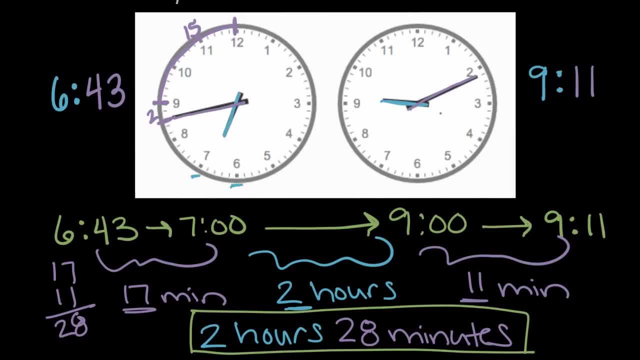 this time on the left, until 9.11, the time on the right.